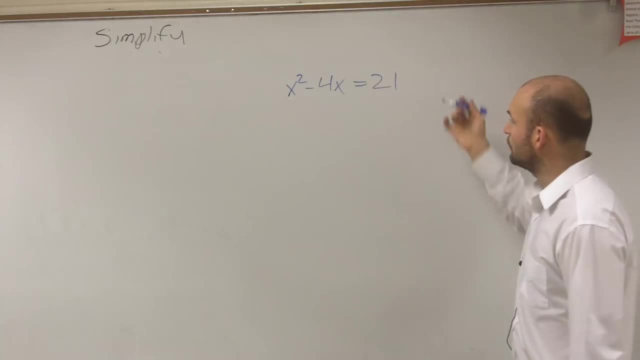 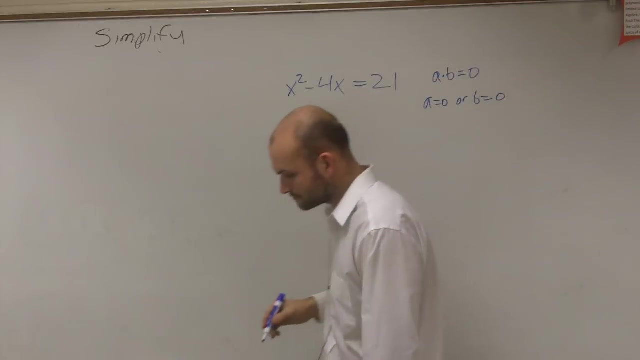 so they're not like terms, We can't just combine them. So when solving for x, we came across this very helpful rule, which is the zero product property, which is any two numbers multiplied, get a view zero. Therefore a equals zero or b equals zero. So what that means. 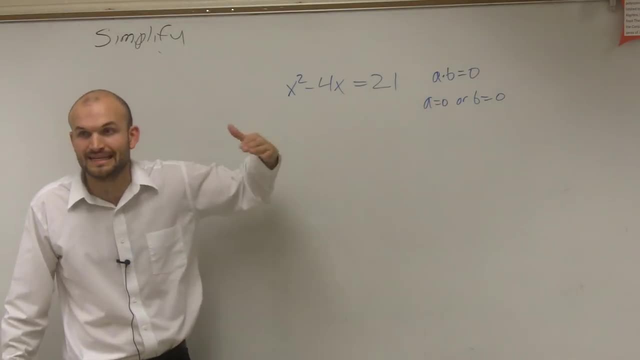 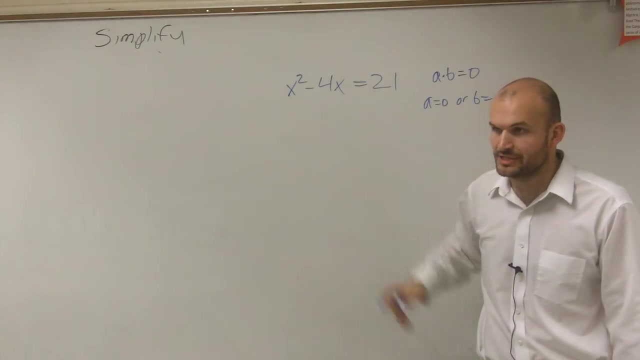 is: if I want to use the zero product property, I've got to have my equation equal to zero. I'll say that one more time, because it's very important To apply the zero product property. you have to have your equation equal to zero. 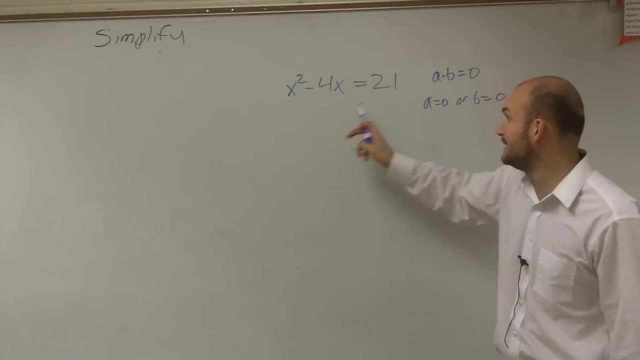 You can't factor this when it's equal to a number. We need it to be equal to zero. So to do that, subtract 21 on both sides. Okay, now can we factor this right? And this is what we've been practicing over and over and over again: right Factoring, factoring. 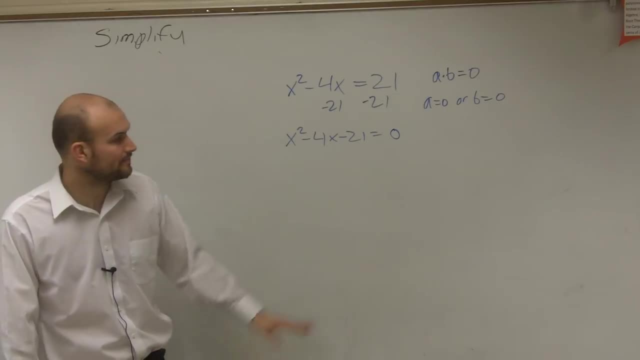 factoring, factoring. So there's a couple different methods. we could do this for You could, like I said, I like to use the x, where you take your coefficient of your square of your first term, multiply it by your last term, which would be negative 21,, and then 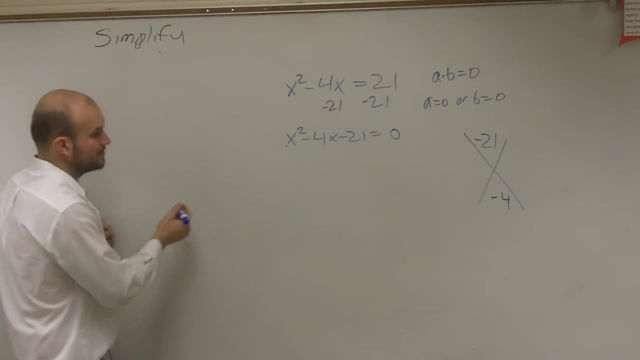 take the coefficient of the middle term, which is negative 4.. Then what you do is you list all the factors of the top and say which two numbers multiply to give you negative 21, but then add to give you negative 4.. So which ones add up? Negative 7 and positive 3, right, 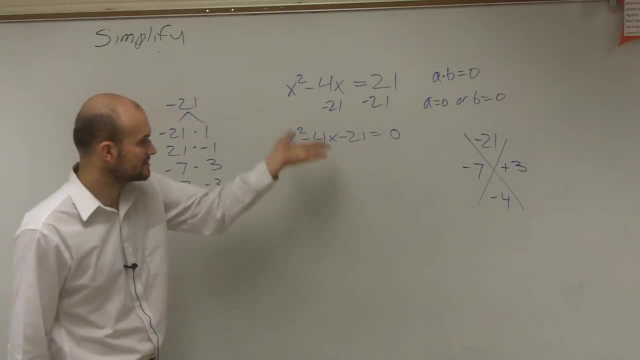 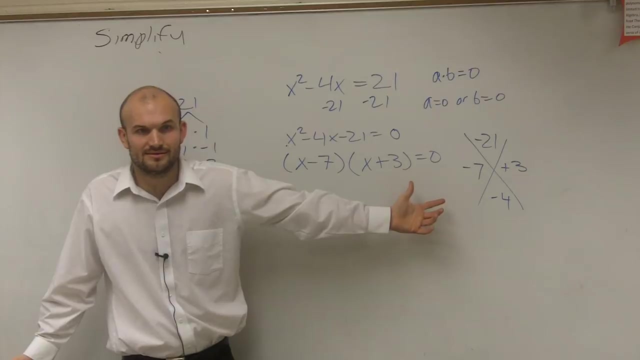 Negative 7 and positive 3.. So then we plug them in Now, do we so? remember, factoring creates a product, right? So now we have a product equal to zero. Isn't that cool, Austin? We have a product equal to zero When you have. 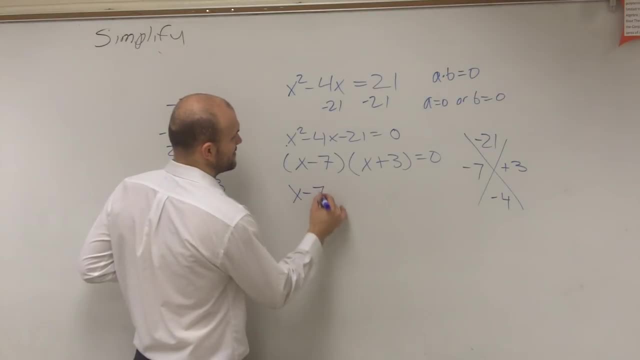 a product equal to zero. you could now say: x minus 7 equals 0, and x plus 3 equals 0.. Therefore x equals 7,, x equals 7, and x plus 3 equals 0.». except that makes nine worldwide. So what I mean is you take the length of n equal to x, you add it up by a fraction. that's not that obvious, but that is n right. So think about it Now, if you have n over n, n over 3,. 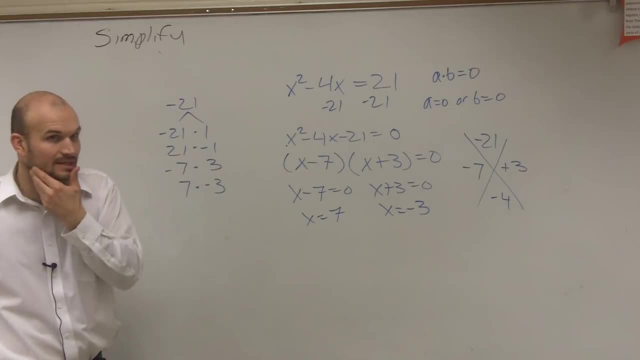 X equals negative 3.. Yes, Could you wait a second? Seems like you're all in a rush.